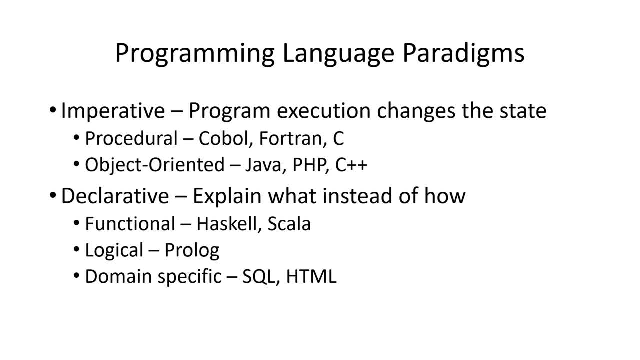 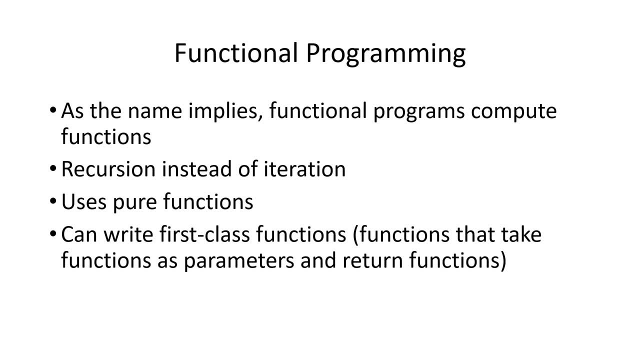 how to do it. It figures out how to do it once you explain what you want. Functional programming computes functions. of course, It uses recursion instead of iteration. Everything is a pure function, which I'll explain in a minute. There are also what they call first-class functions. There are functions. 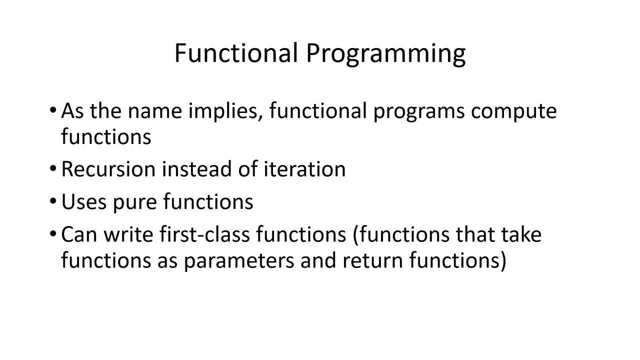 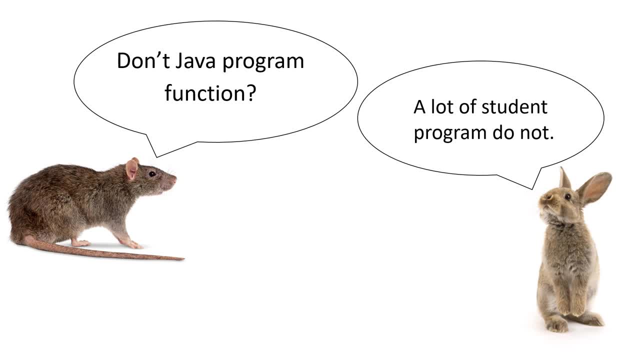 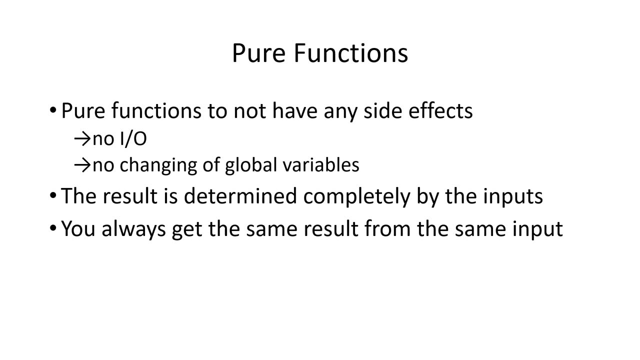 that can take functions as a parameter and return functions. You can't do that in Java. Don't Java programs function? A lot of student programs don't. Can you do it? Of course not. Pure functions do not have any side effects. That is, it acts using the input parameters. 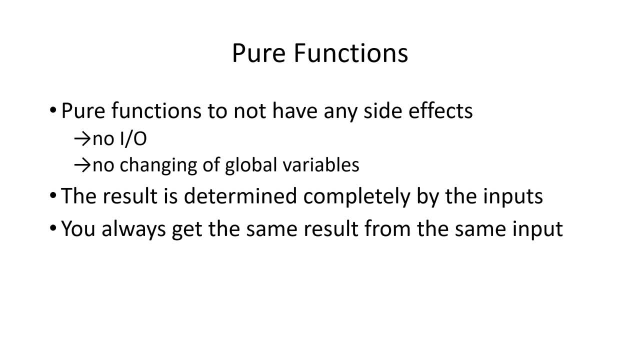 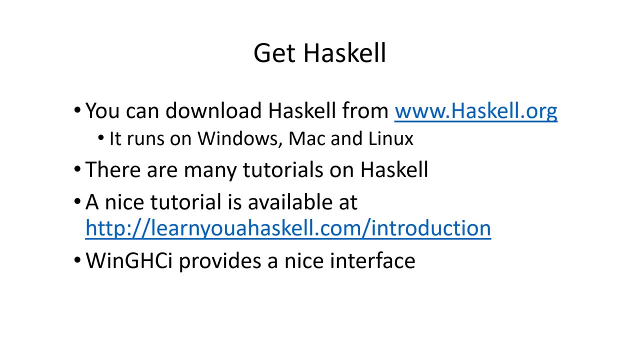 and returns a value changing no global variables. There's no input and output. We'll talk later in a week or so about how you actually read input and output. You should get Haskell and load it on your computer. You can for free from wwwhaskellorg. It runs on Windows, Mac OS X and Linux. I only have a Windows computer. 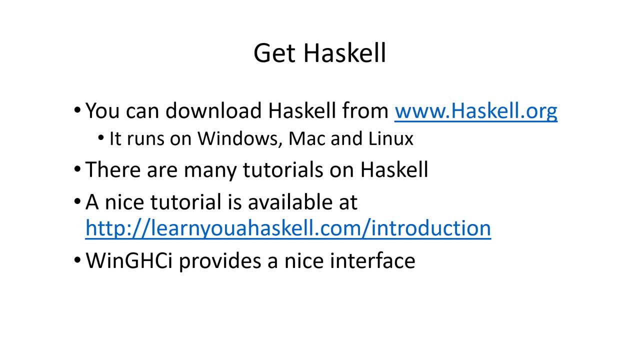 and it works fine on my Windows computer. Somebody with a Mac, please load it and let me know how it runs. There are many tutorials on Haskell available on the web. My favorite one, after looking at several, is learnuhaskellcom, starting with slash introduction And when you download Haskell. 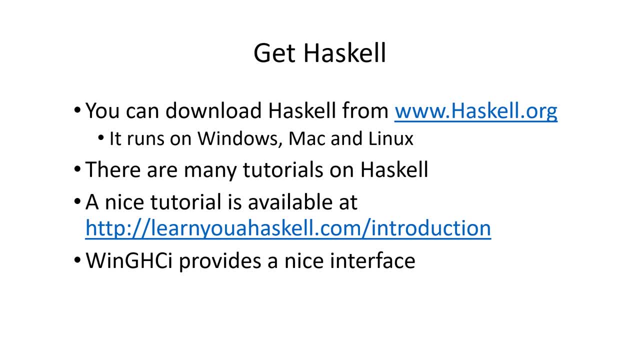 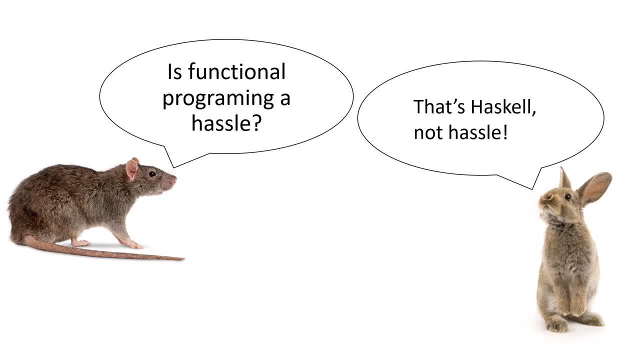 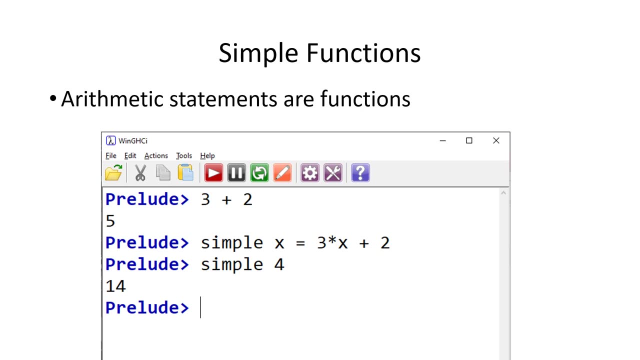 the WinGHCI seems to be the best program to use. Is functional programming a hassle? That's Haskell, not hassle. Clean out your ears In the Haskell system. you can download the WinGHCI program from the WinGHCI website. You can download the WinGHCI. 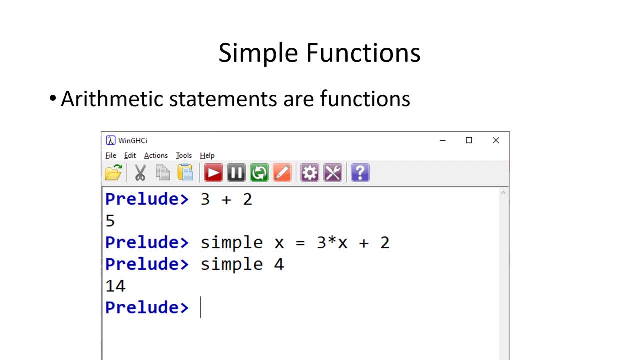 program from the WinGHCI website You can type simple arithmetic statements and they are functions. If you type an arithmetic statement, it returns the result. In fact, in general, when you type a function, Haskell prints the result. So here you can see the example 3 plus 2,. 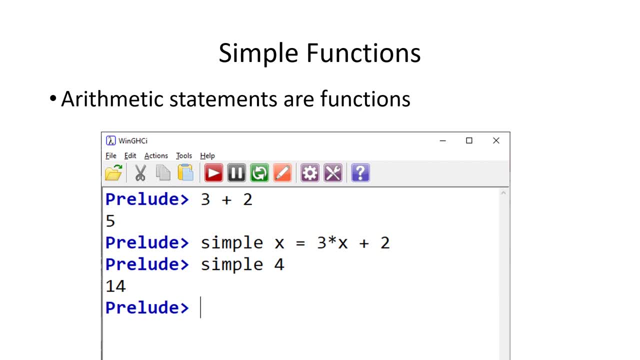 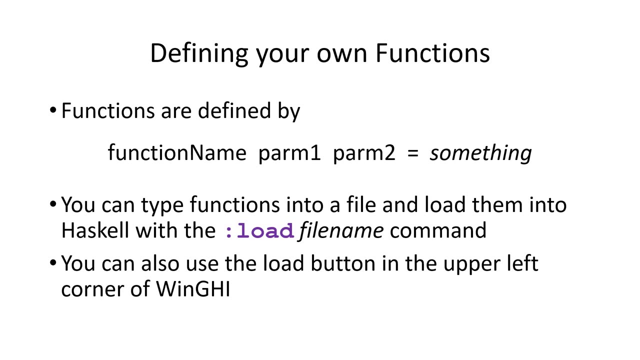 it returns 5.. I can define a simple function which, when you pass a parameter, it returns and prints the result. You can define your own functions in Haskell by putting the function name, the parameters, one, two or as many as you need. 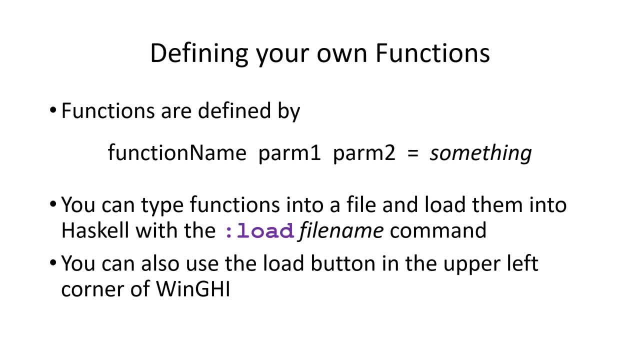 an equal sign, and then the function definition. You can also put your functions into a file and load them into Haskell with the colon load command, Or you can press the button in the upper left hand corner of WinGHCI and then select your file and it will load that function. Note that. 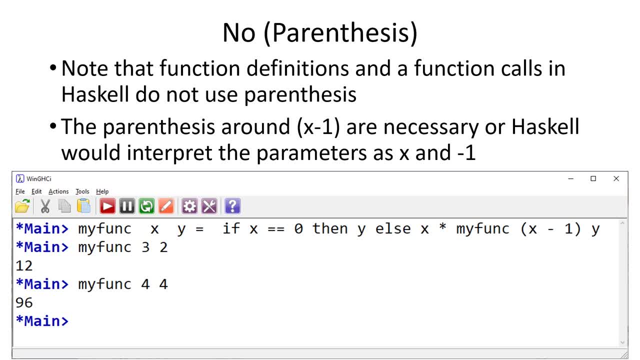 Haskell function definitions and Haskell function calls do not use parentheses. Look at the example below: myfunc- no parentheses there. And then in the definition of the function it recursively calls the function. at the end We have parentheses around the x minus 1.. Otherwise, 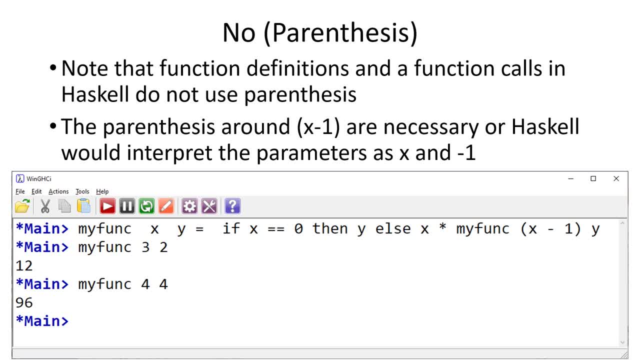 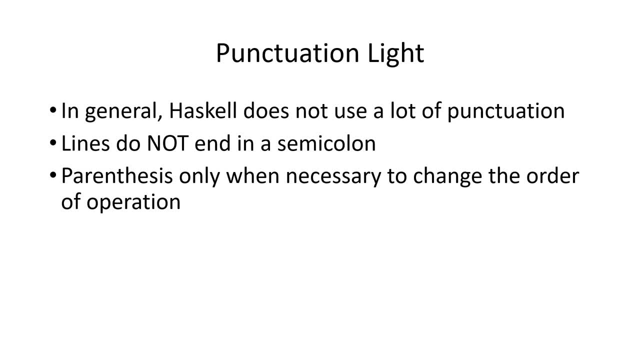 Pascoe would interpret that two parameters to be the x and the minus 1.. In general, Haskell is punctuation light. There are no semicolons at the end and he only uses parentheses when necessary to change the order of operation. If there are no semicolons, how do you know where? 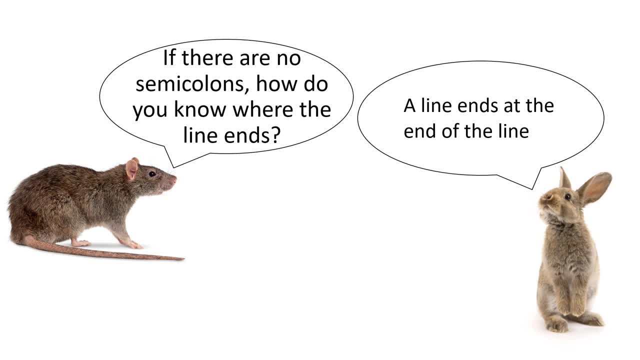 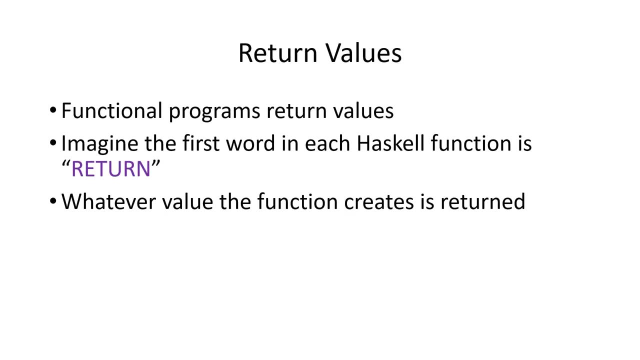 the line ends. The line ends at the end of the line. Each Haskell function is on one line. Functional programs return a value. They have parameters going in and they return a value, No other side effects. You can think of the first word in each Haskell function as being return. 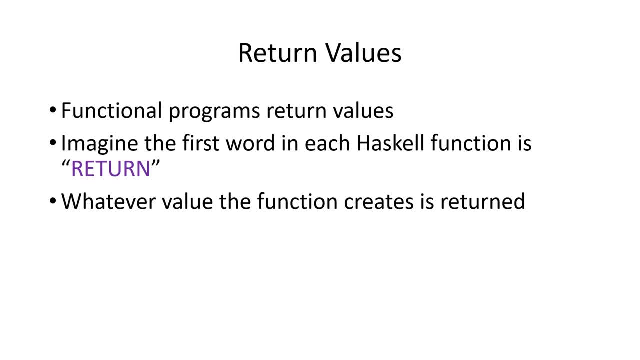 Return this definition, Return the value here. So whatever value a function creates is what's returned. If you're running on the Haskell system, it generally will print that value, although you can call functions from functions, from functions from functions, and it returns those values and uses them. Try writing a Haskell function. 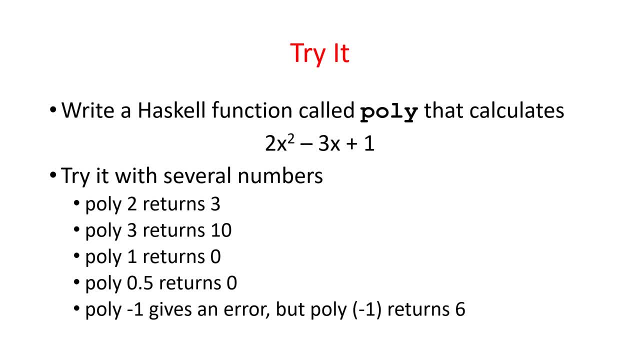 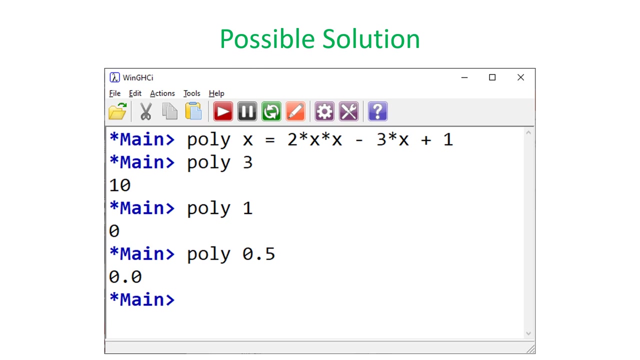 It's a function called poly that calculates the value of this polynomial. So try it now You can pause the YouTube video until you try it. Here's a possible solution. You can say: poly x equals 2 times x times x. we won't go into exponentiation yet. 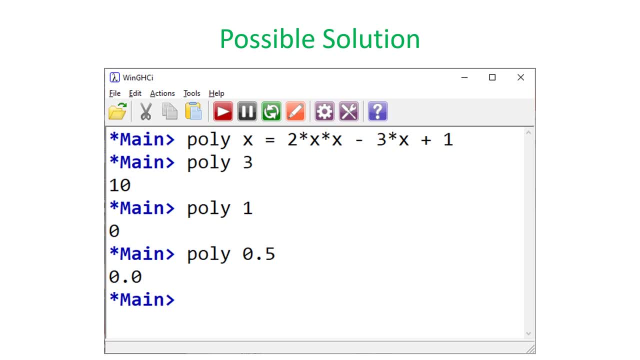 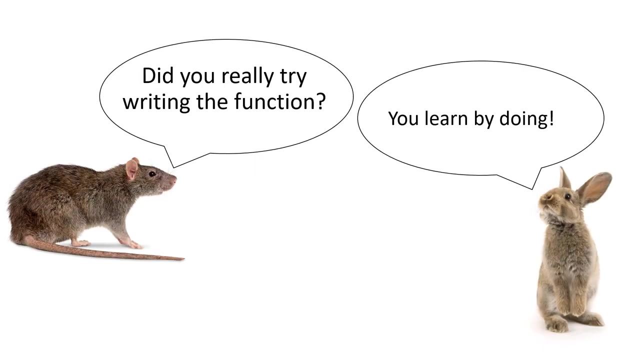 that's 3 times x plus 1.. Then when you call it, you pass it a value that replaces x in the function and calculates that value and returns it, which Haskell system displays it. So the poly of 3 is 3 times 3 equals 9, times 2 is 18, minus 9 plus 1 equals 10.. 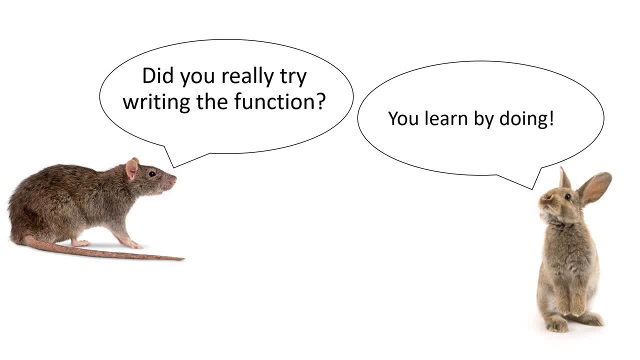 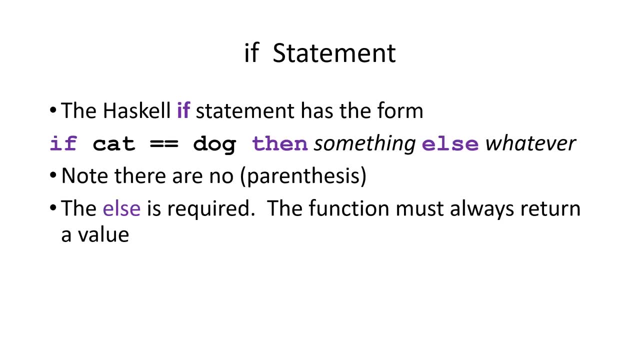 Did you really try writing the function? You learn by doing, Don't you? I'll do that again in 5 or 10 minutes. Bye, just try to listen to old Dr Williams, The Haskell. if statement has the form, if a comparison, 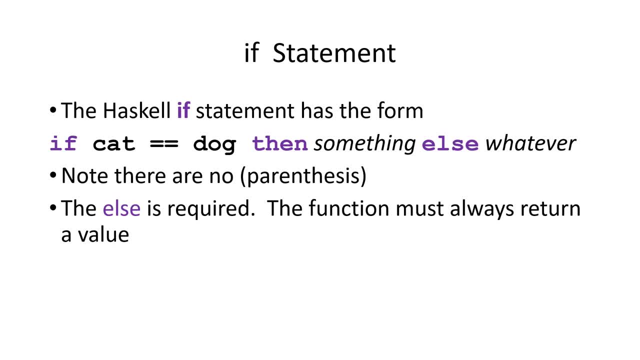 expression or a logical expression, then something else, something else. The comparisons are just like they are in Java or C, where double equals is equals, or you can have greater than or less than, or less than or equal. to Note, there are no parentheses. Else is required. 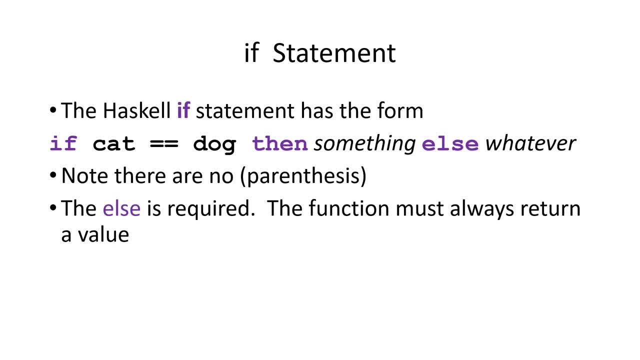 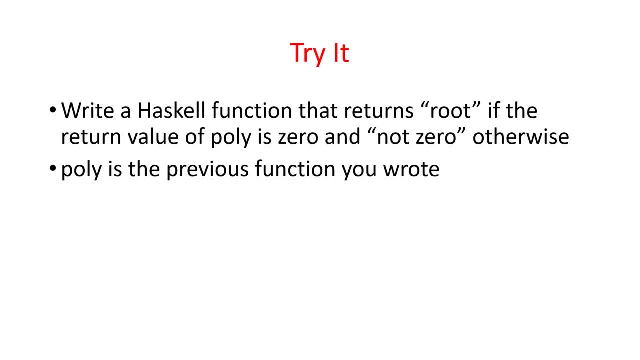 You have to put the word then and the word else in there. You got to have an else because functions always return a value. If you had a then and there was no else, it wouldn't have anything to return. So try writing another Haskell function that returns the word root. 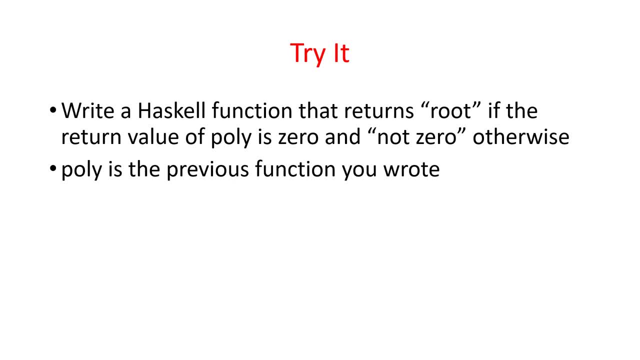 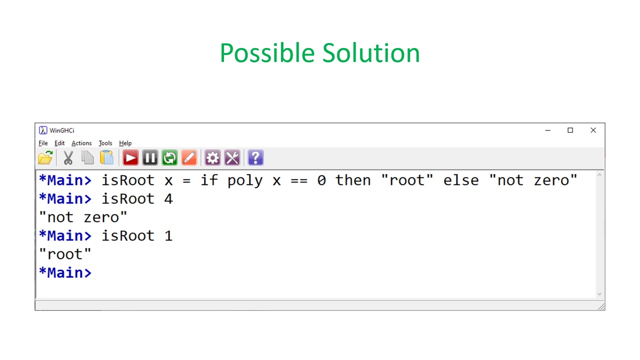 if the return value of the previous polynomial function is zero and nothing else, not root. otherwise, Pause the YouTube video and give this a try. Here's a possible solution We go is root x equals, not equal means the definition of the function. then we have: if poly x, poly being the previous function we wrote, if that's,